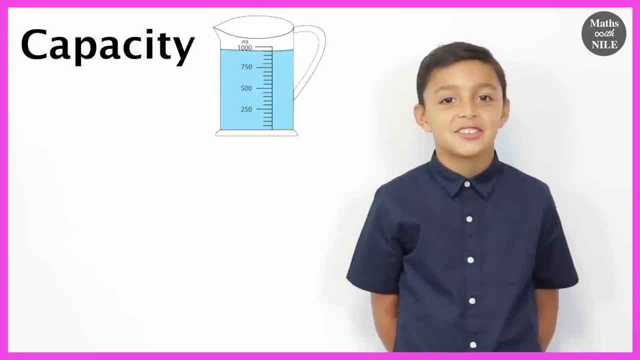 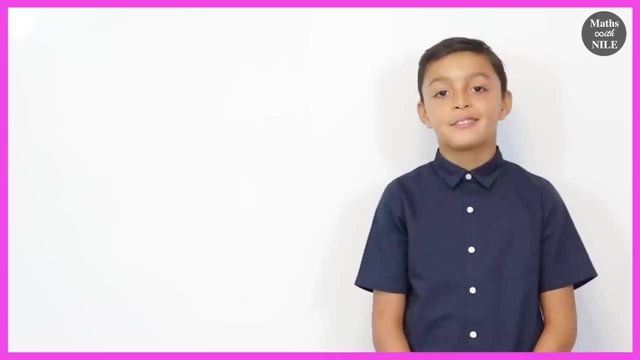 Capacity, Capacity And what is capacity? measured in Millimetres or litres, And how many millimetres in one litre? One thousand? I'm going to ask you a few questions, Niall, and I want you to tell me what is the best measure. 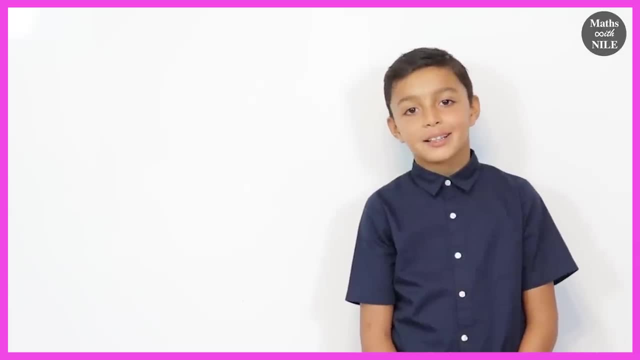 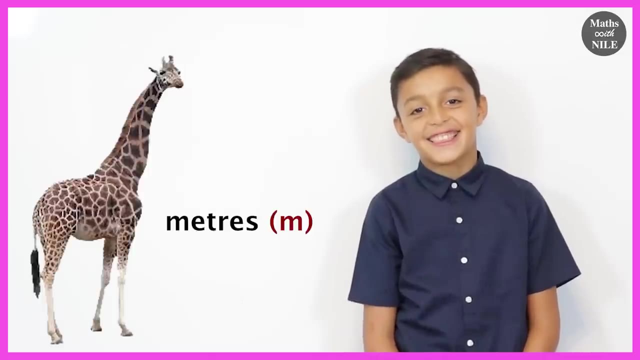 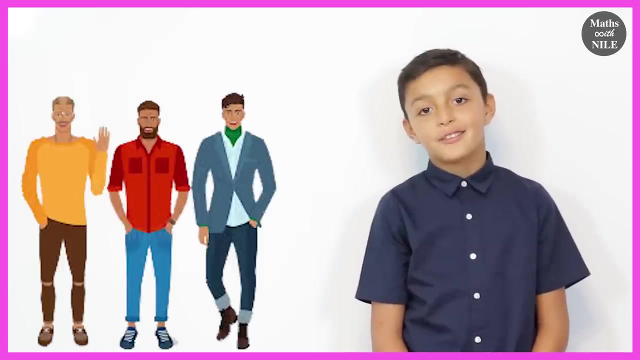 for each of these. Okay, Are you ready? Okay, the height of a giraffe: Metres, Okay, metres. What about the mass of a man? Kilograms, Kilograms. Niall, do you know what your mass is? 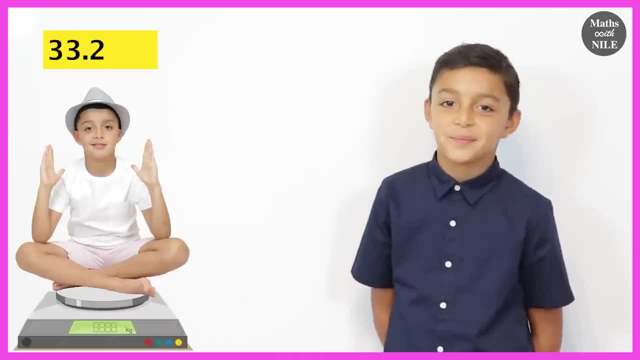 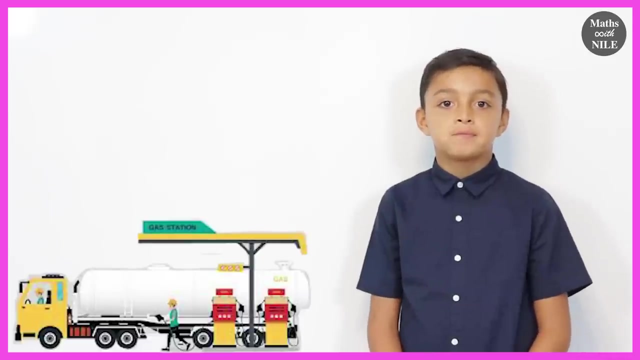 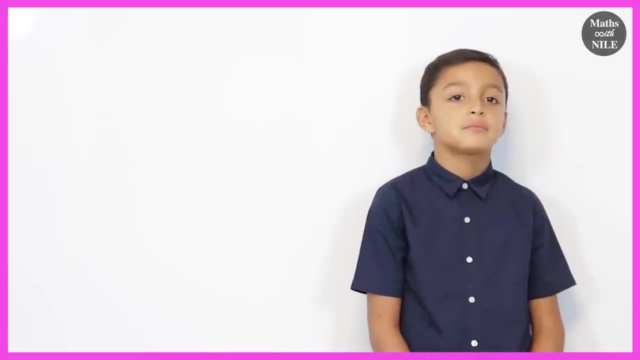 I think I'm thirty-three point two: Kilograms, Kilograms. And how do you know that I read myself earlier. Okay, What would you use to measure how much petrol to fill a truck? Litres, Very good litres. What about the mass of an orange? 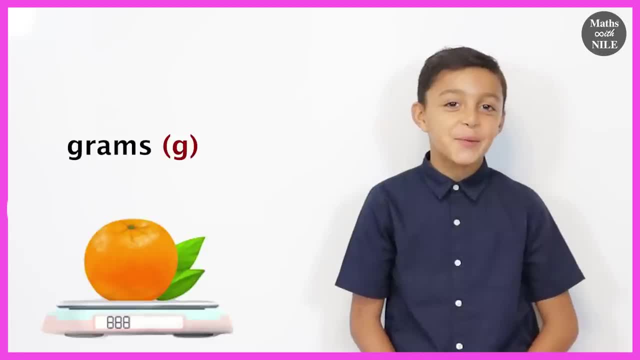 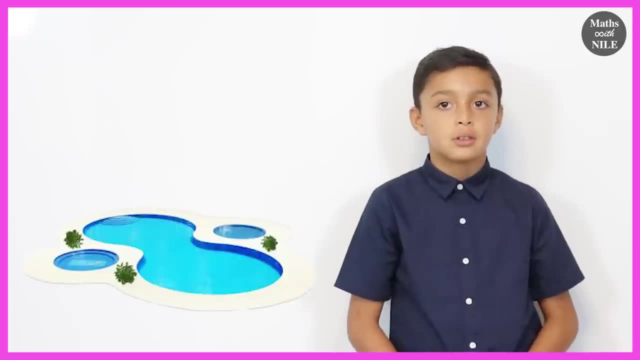 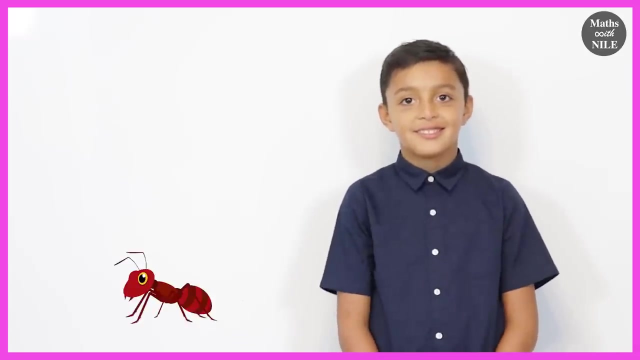 Grams, unless it's the world's biggest orange. I would stick with grams, I would, Okay. What about the amount of water in a swimming pool? Litres, Litres. The length of an ant: Millimetres, Millimetres. 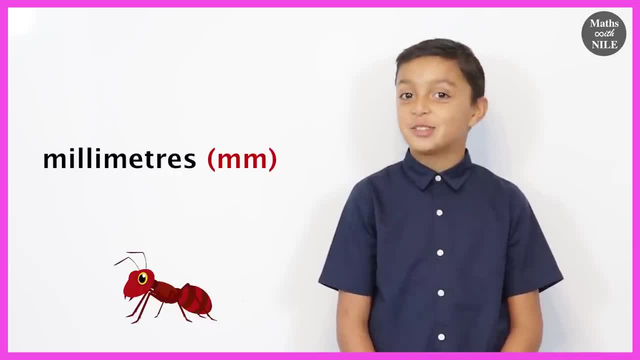 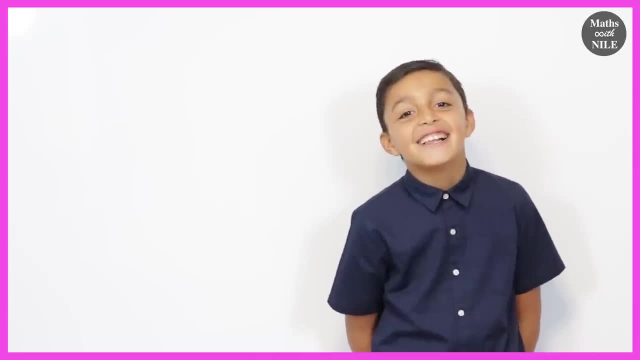 I don't think millimetres would work. I think millimetres are too big still. We are not going to test that one, I'm afraid. What about the distance from England to France, Kilometres, Okay. What about the mass of a table? 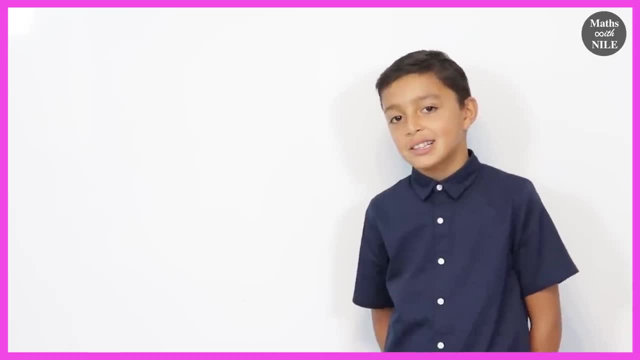 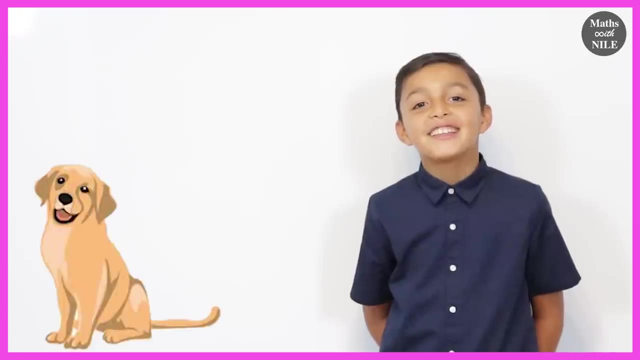 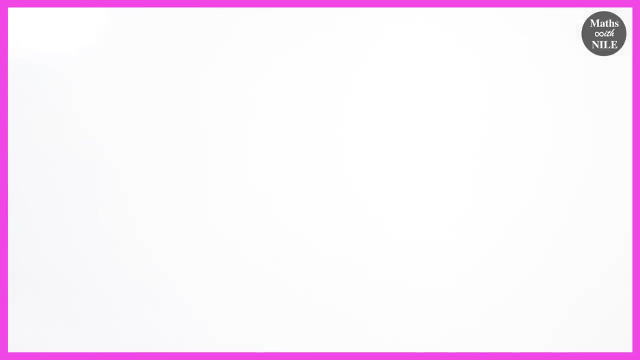 Kilograms, Kilograms. What about the length of a dog? I see you're looking at your dog. Why don't you pick him up and then we'll have an idea. We all know, Frankie, unless you're new. We all know, Frankie. 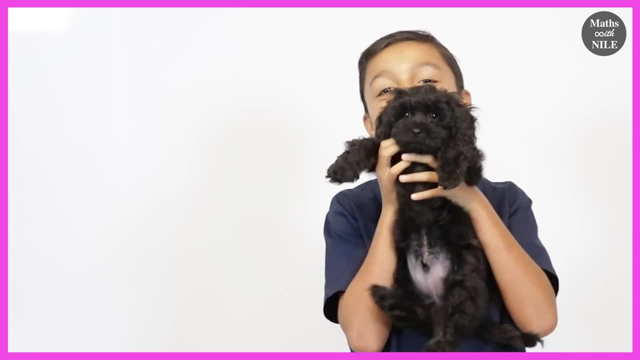 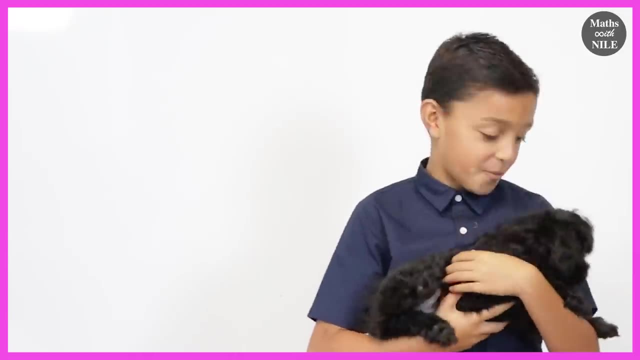 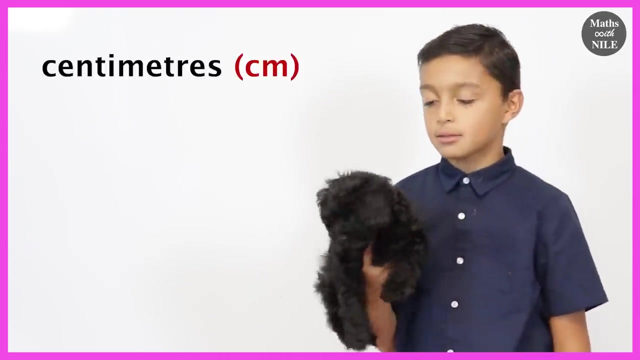 but I got a new dog. What's your dog's name? Milo? Okay, So, Milo. So what would you use to measure the length of Milo Um centimetres, Centimetres? And what about your height, Niall? 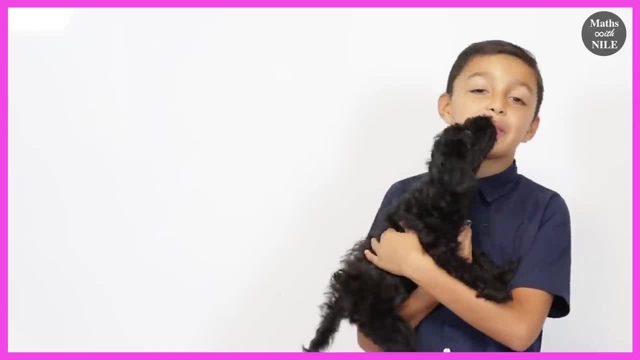 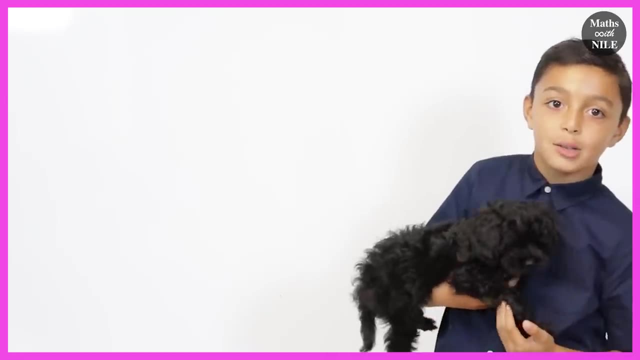 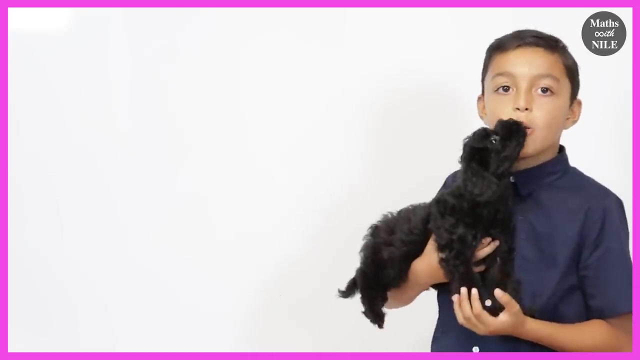 Metres. Well, it could be metres, or it could be centimetres, because I'm one meter, point four, something centimeters. so how do you say it? one? if you say it in meters, what would you say? 1.4 meters? okay, and in. 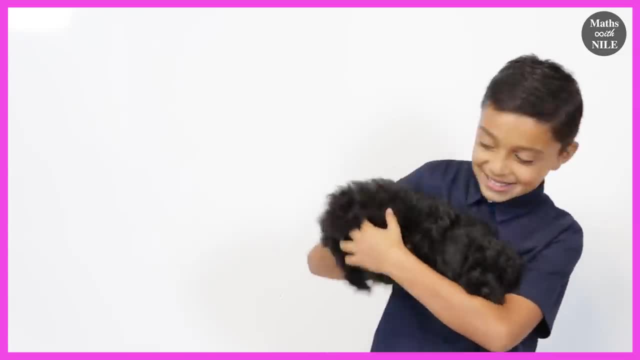 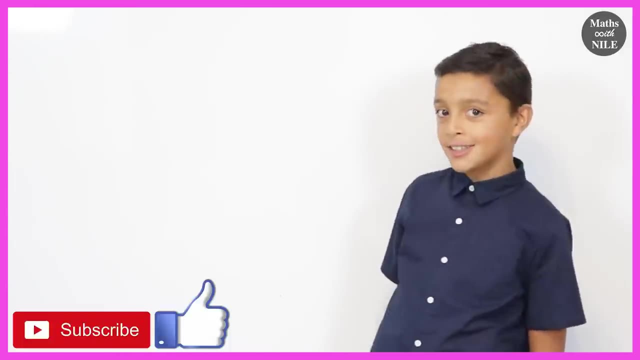 sense, 140 centimeters. okay, good, if you're enjoying that video, don't forget to smash that like and subscribe button and look out for the next videos, because we'll be measuring length, math and capacity, lovely Nile. before we finish today's lesson, though, I have a few questions for you, so a little bit of a. 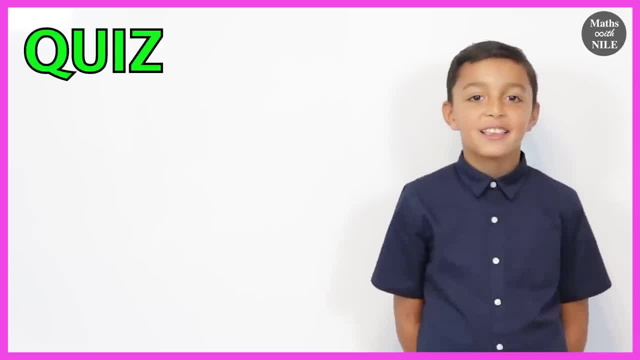 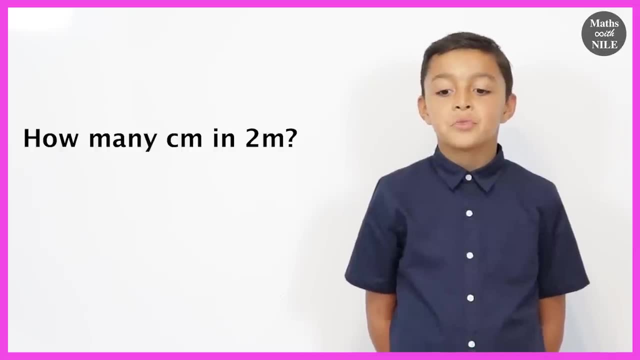 quiz. are you ready for this? okay, now. can you tell me how many centimeters are there in two meters? 200, 200 centimeters? how many milliliters are there in 3.5 meters? how many milliliters are there in 3.5? 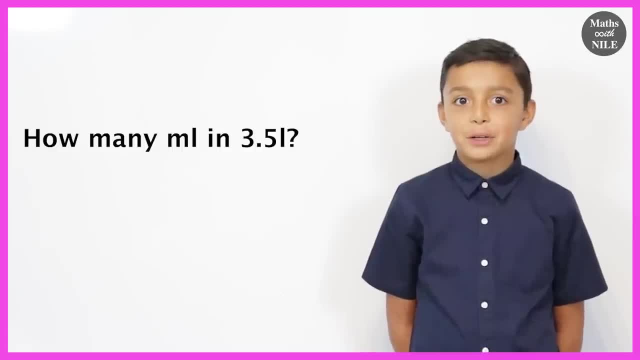 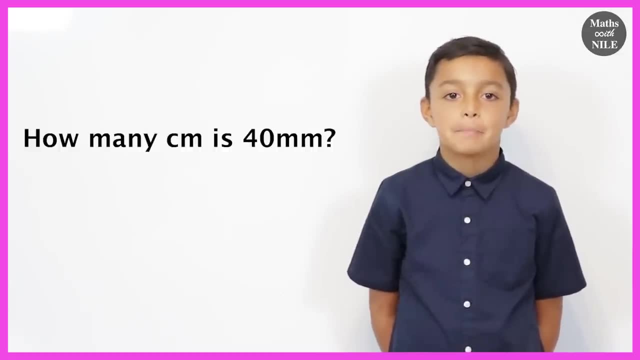 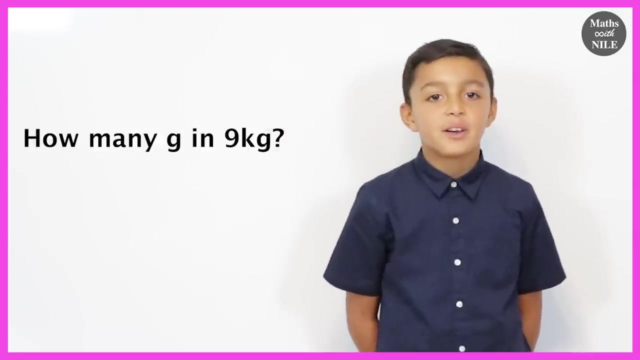 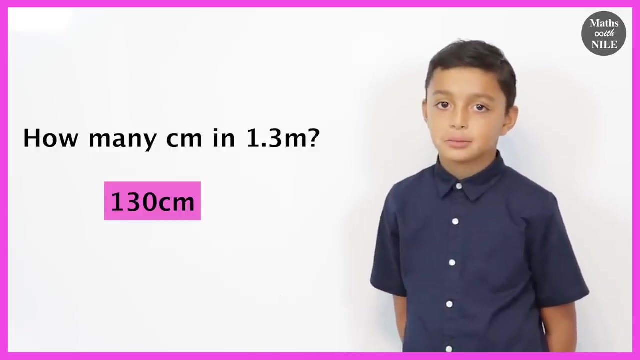 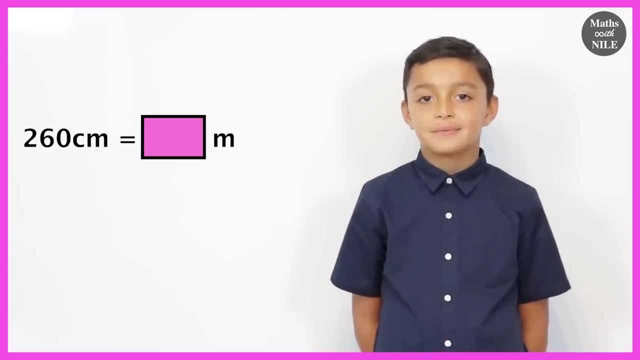 meters? how many centimeters is 40 millimeters? how many meters in four kilometers? good job. how many grams in nine kilograms? how many centimeters in 1.3 meters? last question, 260 centimeters is how many meters 2.6, 2.6 meters, and that's how many centimeters are there in 1.3 meters? 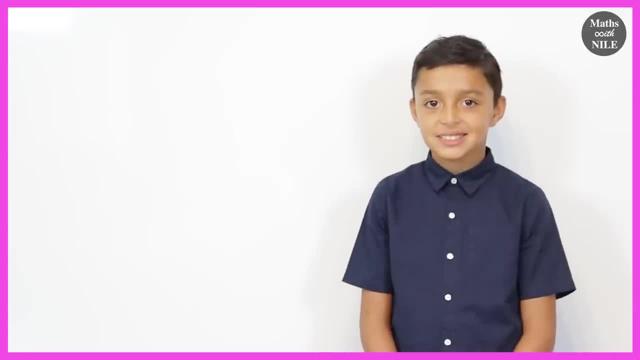 how many centimeters in 1.3 meters is how many meters? 2.6 meters and that's how many centimeters are there. and that comes at the end of today's lessons, by enjoy the video and issue those with right now.